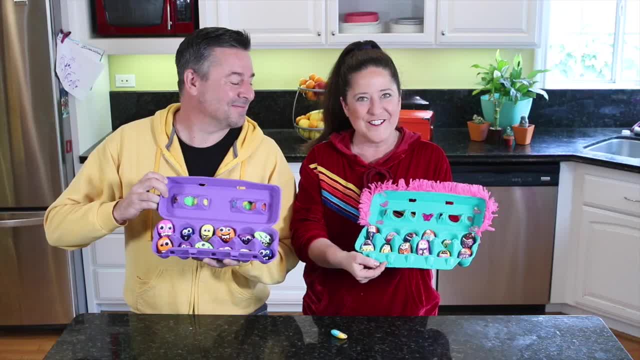 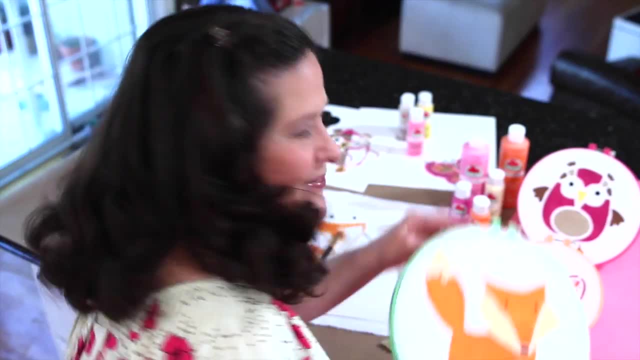 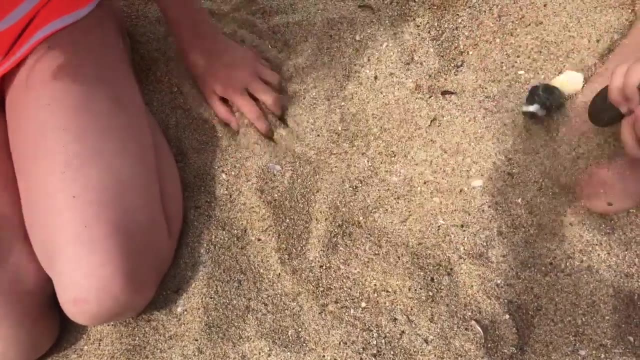 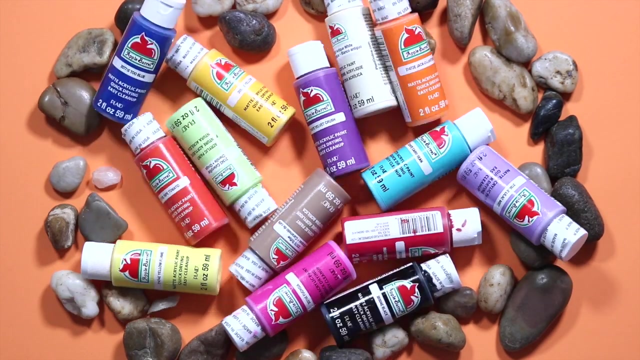 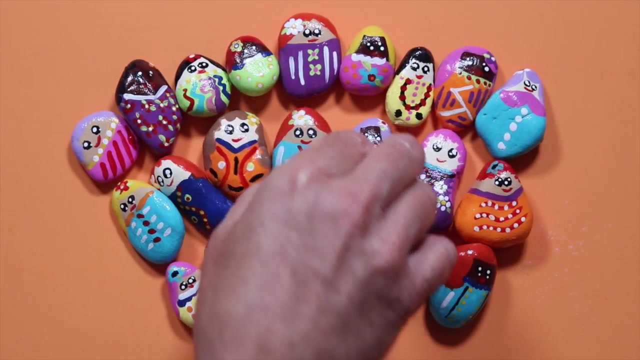 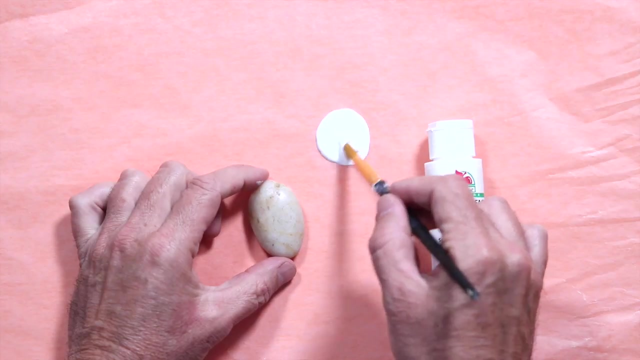 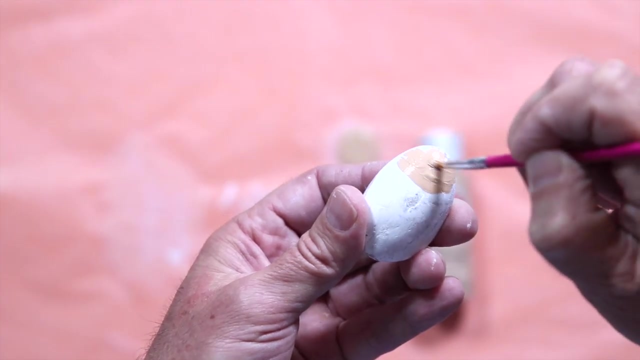 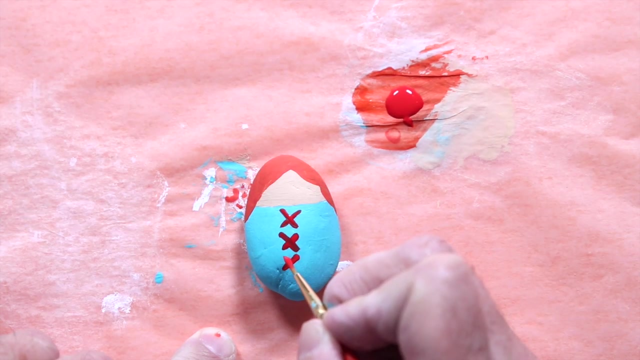 I made a jewel encrusted one to house all of our little dolls. Kathy, are you ready to do this? Let's do it. Hurry, we need to make it. GYeah, Do we See how easy it is? 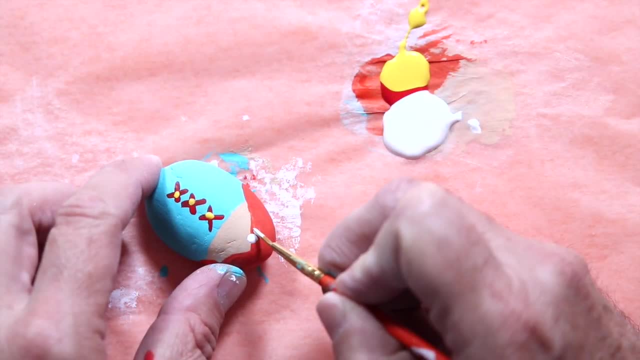 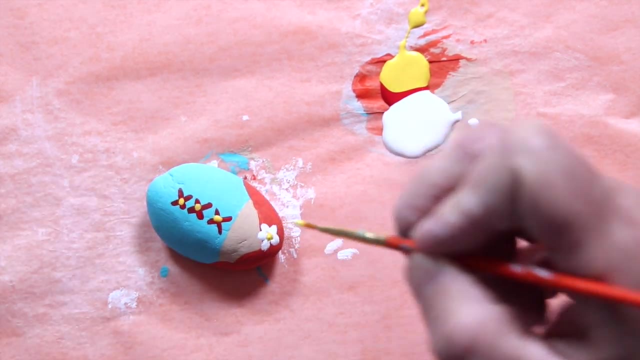 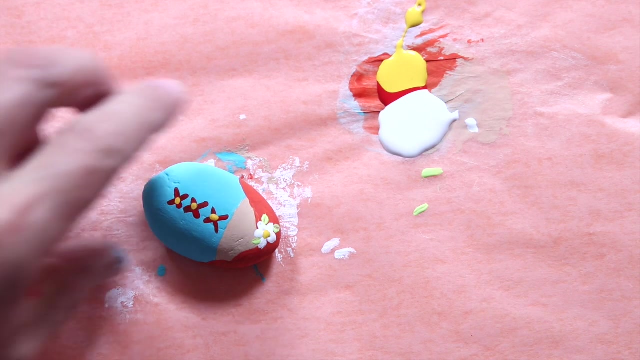 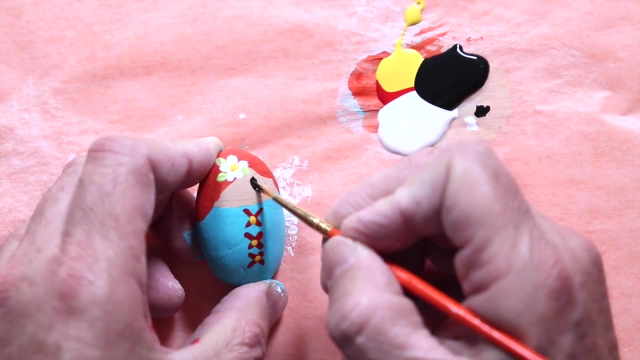 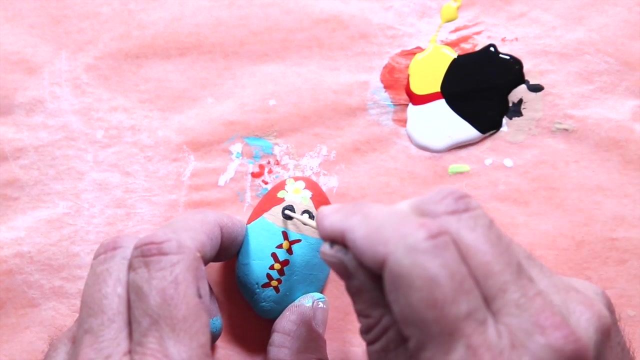 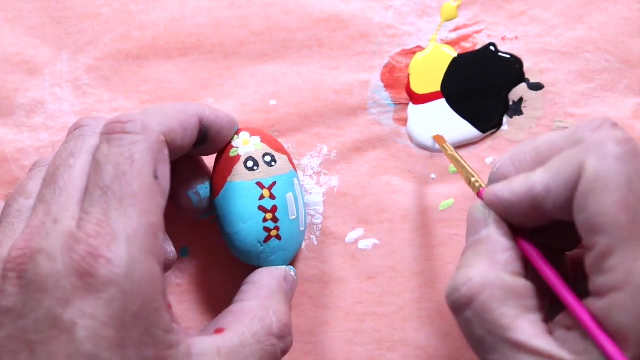 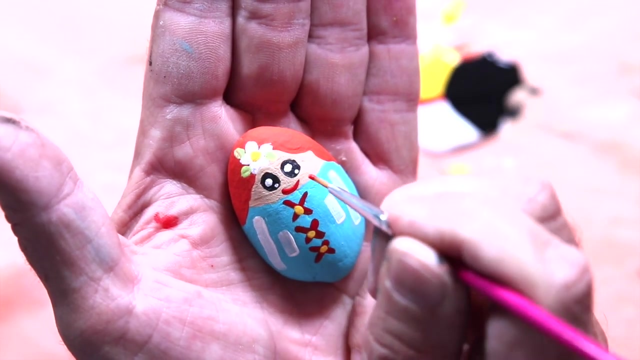 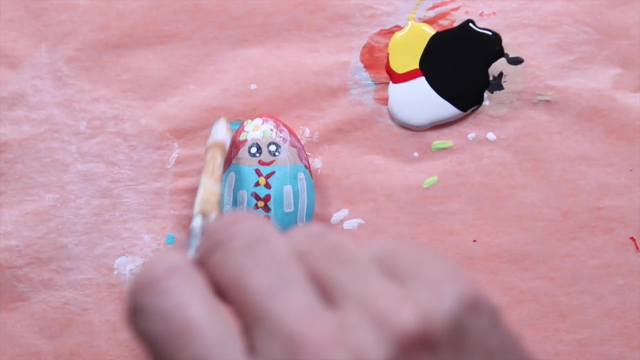 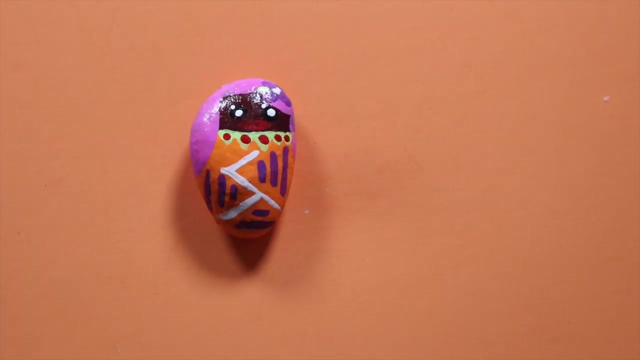 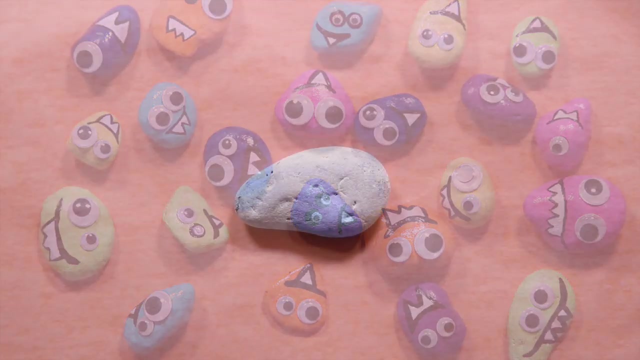 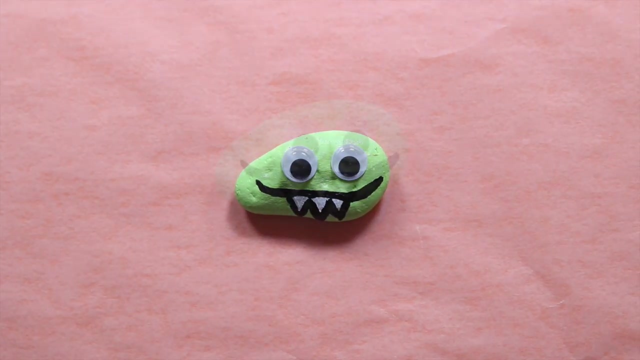 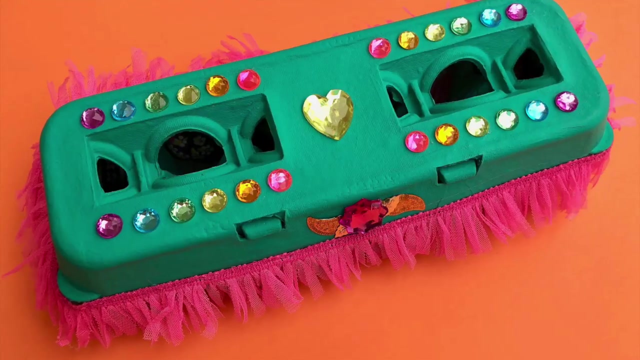 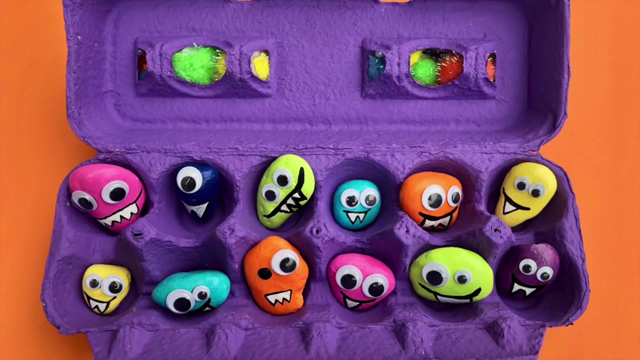 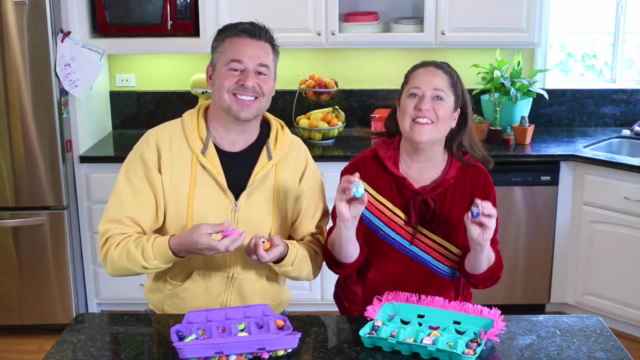 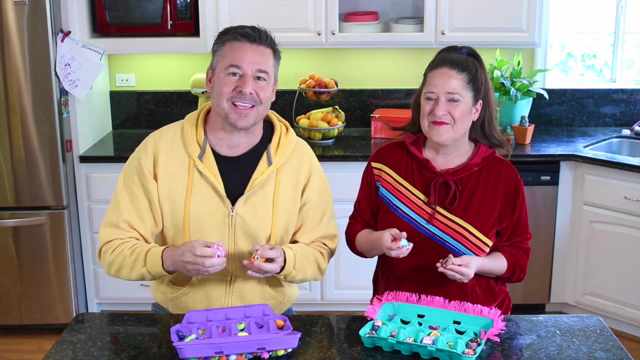 Cheers Thanks. Thank you for watching. Thank you for watching. Thank you for watching. I cannot pick a favorite. I love them all so much. I know These were super fun to make and so easy. It's very simple. We hope you create some painted rocks with your family this weekend. 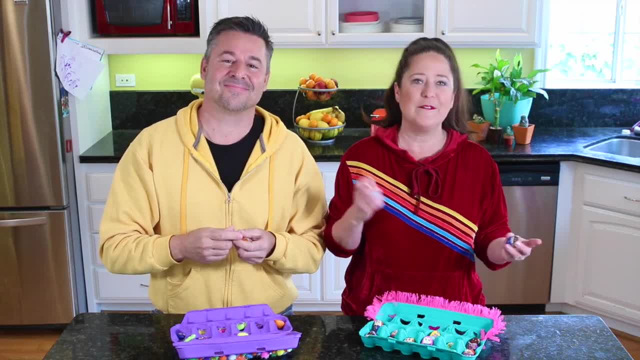 And if you do, be sure to tag Plaid Crafts Like share, drop us a comment. We will see you next time on Family Craft Night. Bye, guys.